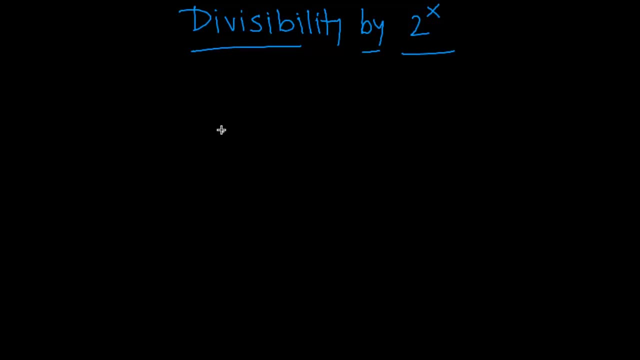 In this video, I am going to teach you how to see if a number is divisible by 2 or any powers of 2, like 2 square or 2 cube or 2 raised to x. Now, almost all of us know this thing and still just revise it. 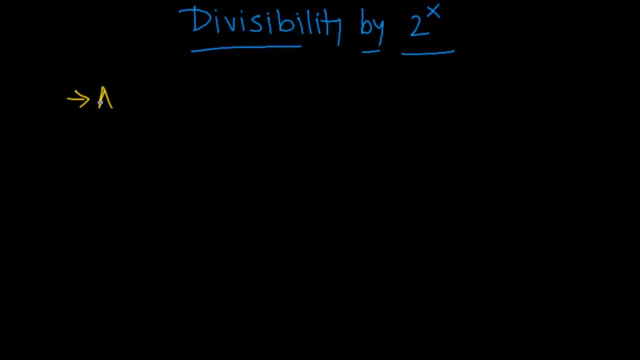 Any number that ends with even number is divisible by 2.. So basically, any even number would be divisible by 2.. So, for example, if the given number is 14, you can simply look at this unit's place and say that if unit place is 4,, that is, unit place is divisible by 2, then this entire number would be divisible by 2.. 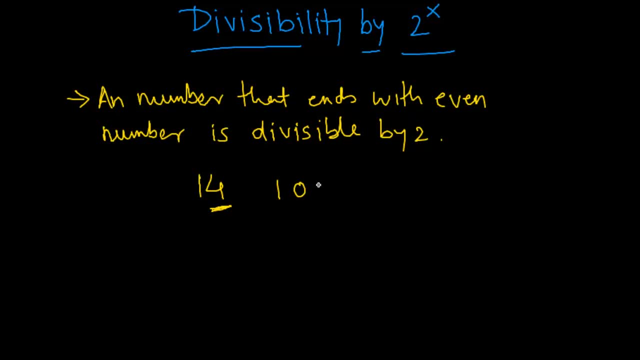 If you are given the number like 101691, without even dividing, you can straightly tell that this number won't be divisible by 2 because the unit's place is odd-digit and hence the number won't be divisible by 2.. But obviously there has to be some logic why this method is working. 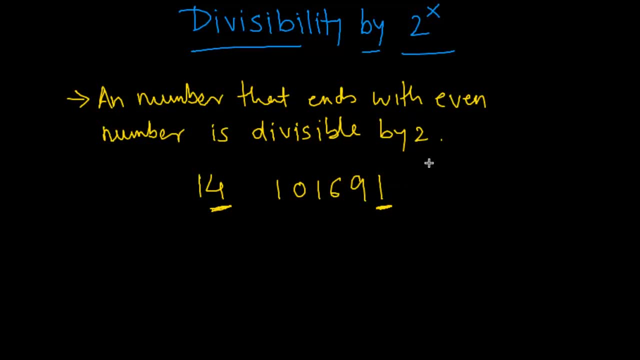 So let us understand this logic first, And based on this logic, we are going to derive the divisibility for 4,, 8 and 16 and so on. That is for any 2 raised to x thing. So now for any number. 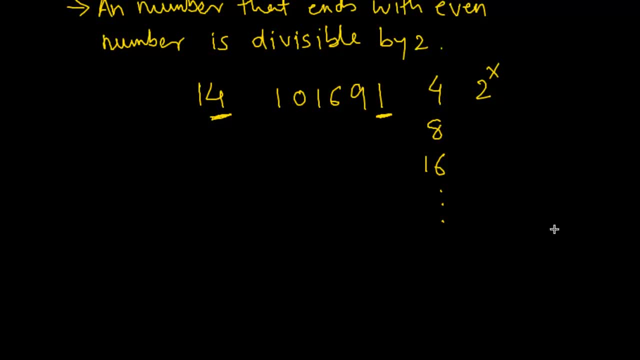 To be divisible by 2,, it should be multiple of 2.. See- let us take this example again- 14.. Now why 14 is divisible by 2? Because it is 7 into 2.. So it consists 1, 2, and so it would be divisible by 2.. 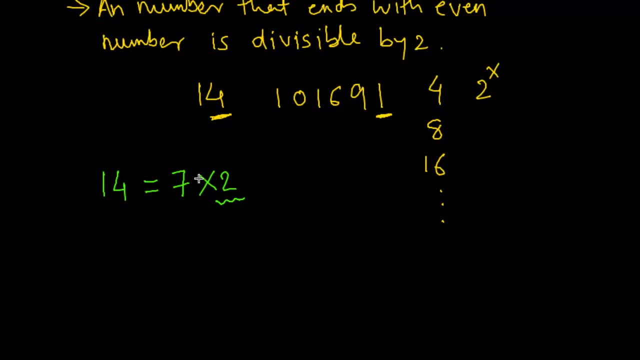 And why this won't be divisible by 2 is because when you will write its standard form, that is, or when you will represent it as a multiple of it, some prime factors- you won't be able to find 2 in it, Like, say, suppose, 37.. 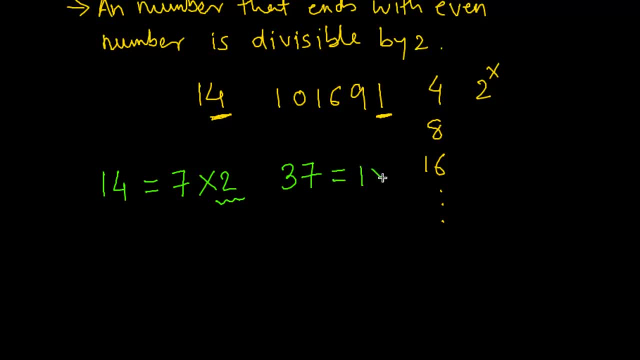 Now, 37 itself is a prime number, So you won't be able to divide it by 2, because obviously 2 won't be its factor. Now let us say 33.. Its unit place is 3 and this number won't be divisible by 2.. 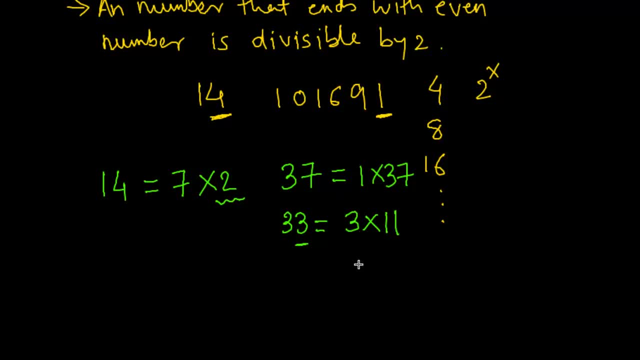 Why? Because 3 into 11 is 33.. 3 into 11 is 33. And in standard form it really does not have any 2.. Now let us think, just ponder over it a bit, Why divisibility simply is dependent on its unit digit. 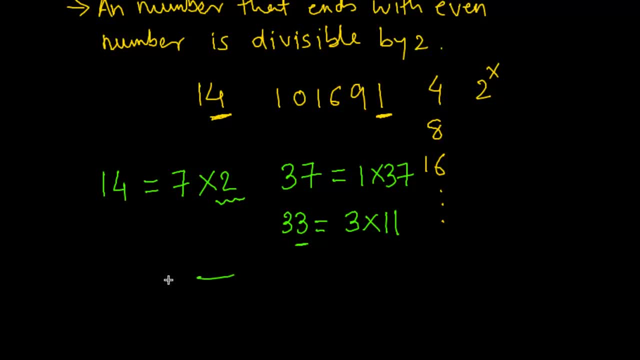 That is just because suppose this is 1's digit, Here the unit digit, tenths, hundredths and whatever, Now all the tenths, all the hundredths and all the thousands would be divisible by 2.. That is because, suppose the number is 10.. 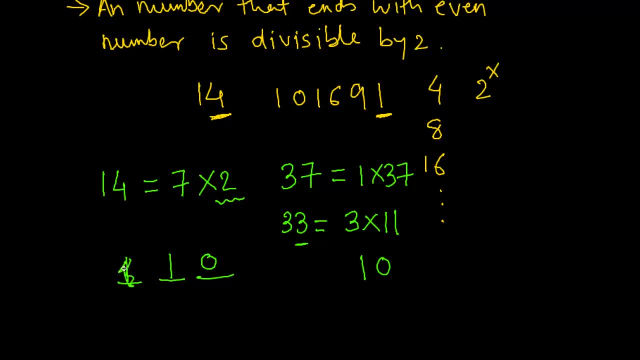 We are assuming 0 at the unit's place And this place does not exist for now. So 10, it will always have 5, 2 into 5.. That is 5 into 10 and it will always have 2.. 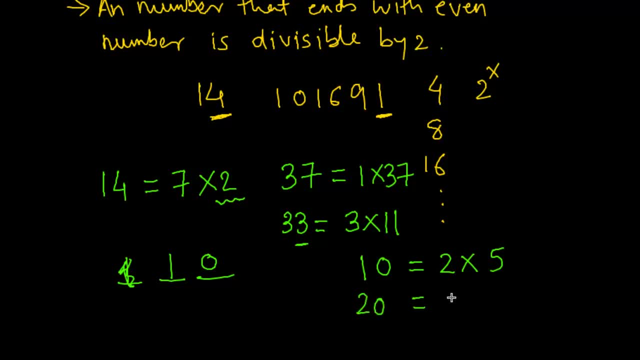 If the number is like 20, it will always have 2 into 2 into 5.. If the number is 30, it will always be divisible by 2.. That is because 2 into 3 into 5. So it will always have 2.. 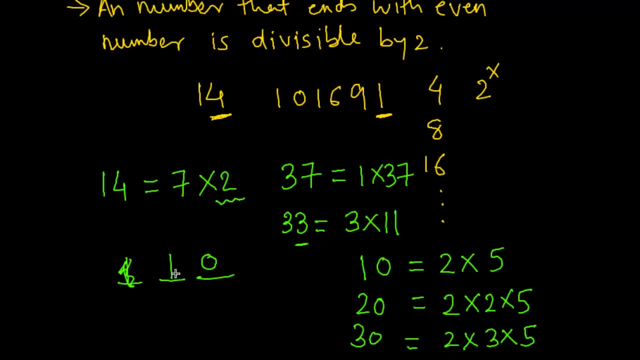 That is because. so what it effectively means is that all 10's are divisible by 2. no matter what number you place over here, That part is always going to be divisible by 2.. So only individual part would be in its place. 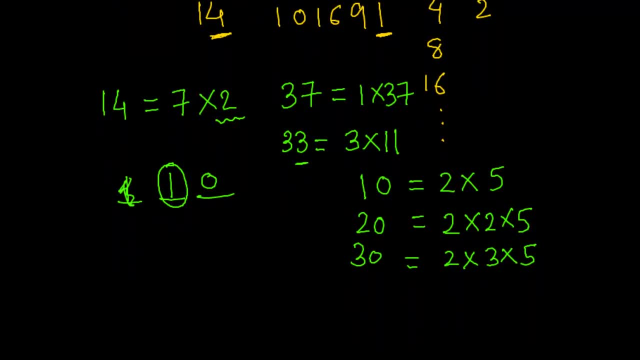 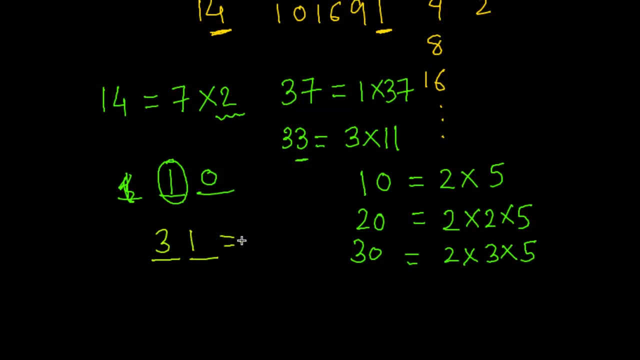 Divisibility by 2 heavily depends upon the unit's place. See, when you write 31,, you effectively mean that it's 30 plus 1.. Now this part is obviously going to be divisible by 2.. The thing that is not divisible is: 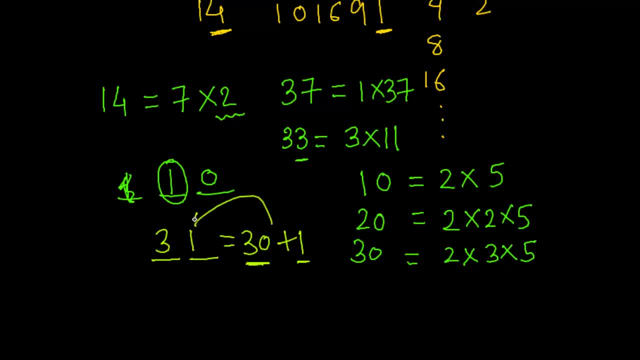 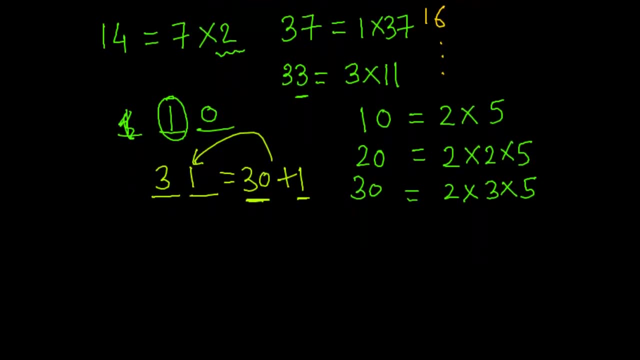 this one, And hence we always rely upon the unit's place of a number for divisibility by 2.. So that was all about 2.. Now let us talk about 4.. Let us talk about number 4. That is, 2 squared is. 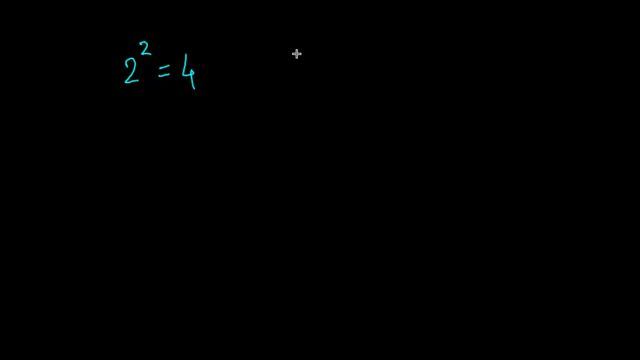 4.. Now the method to know the divisibility by 4 is for any number. let us say 124.. If the last two digits are divisible by 4, then the entire number will be divisible by 4.. So here, 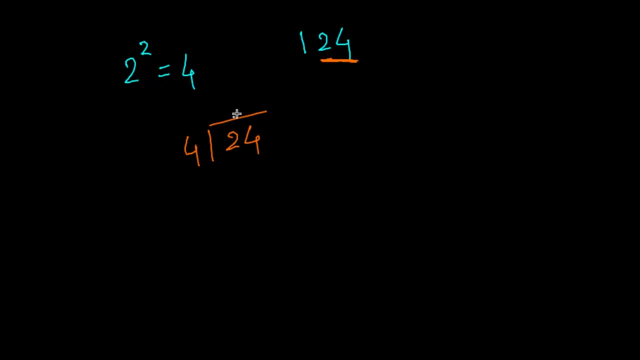 24, 4, sixths are 24.. And we get 0 as a reminder. So 24 is divisible by 4, and hence 124 should also be divisible by 4.. So 24 is divisible by 4, and hence 124 should also be divisible by 4.. 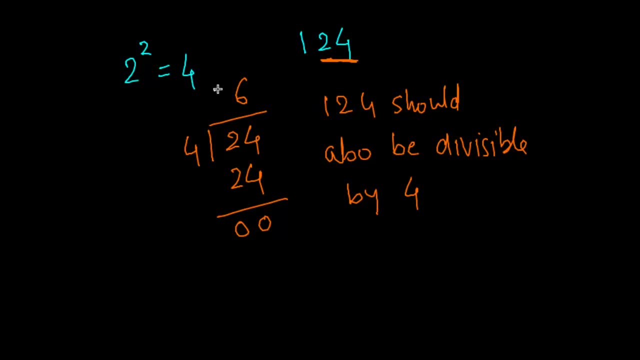 Let us understand about this: 4.. So now, how will you write it? 100 plus 24.. Now, all hundreds are always divisible by 4. Be it 100, be it 200, be it 300.. If a number given is 232,, 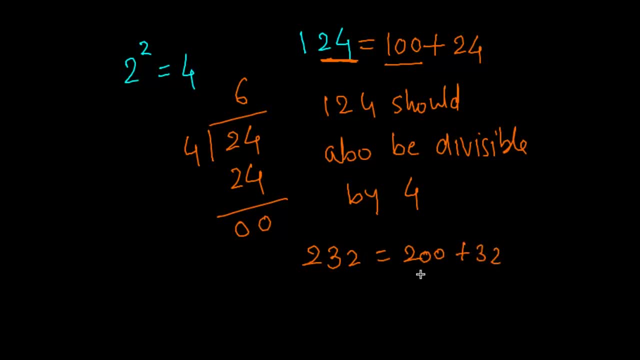 then it will be 200 plus 32.. Now, 200 is obviously going to be divisible by 4.. The only thing that is not going to be divisible is this part: Suppose a number- here- 32- is divisible by 4.. But if a number given is 231, then what? 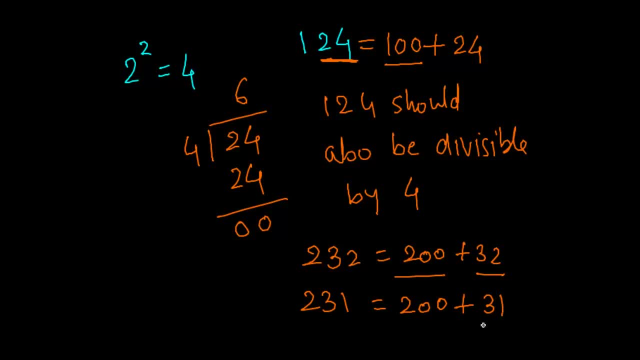 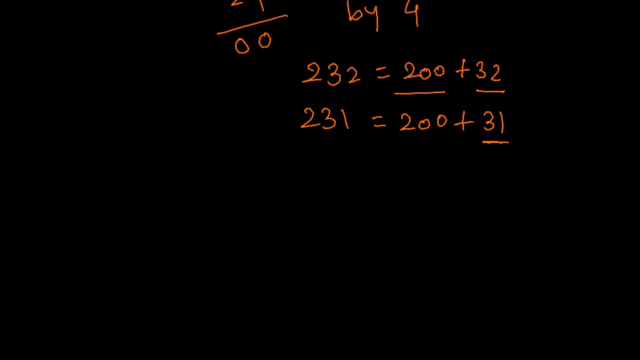 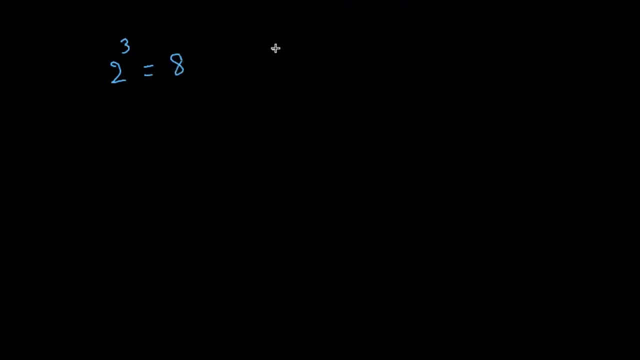 What is the next power of 2? 2 cube? What is the next power of 2? 2 cube? What is the next power of 2? 2 cube? 2 cube, 2 cube, That is 8.. 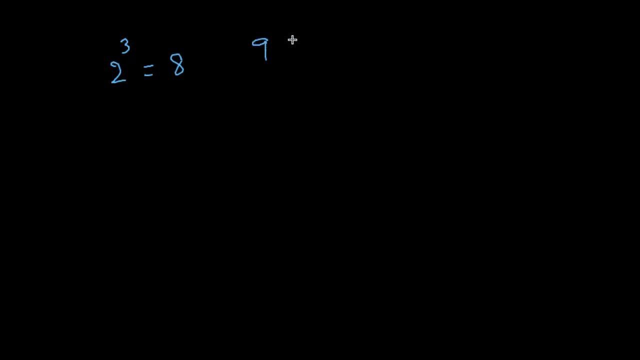 Again, suppose the given number is 9653.. Again, you will be in doubt. how to know? First, just simply divide it by 8 and see. Other thing is see the last three digits. Why last three digits? Because all the thousands would be divisible by 8.. 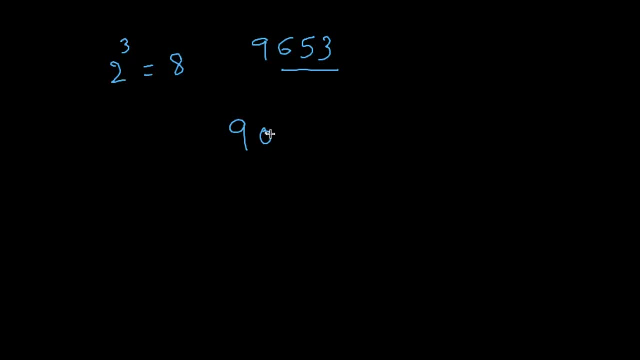 Now why all the thousands would be divisible by 8?? See, the number given is 9000.. It is kind of thousand. All the other places are zero. See, the number given is 9000. It is kind of thousand. All the other places are 0.. 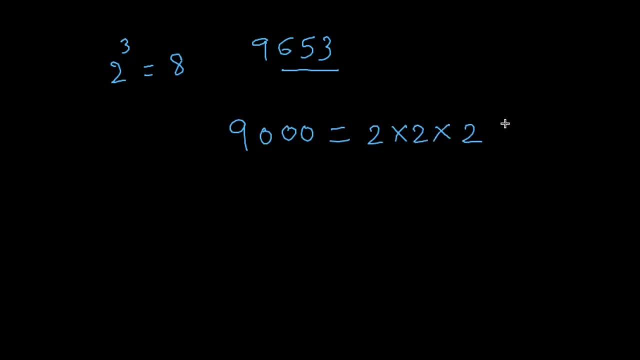 obviously have three, twos in its prime factorization and dot, dot dot say simple number, thousand. then we can represent it as a two into five hundred, that is two into two, into 250, that is two into two, into two, into five, into five, into five, two to the four, four to the eight, eight by the forty, two hundred in thousand. so 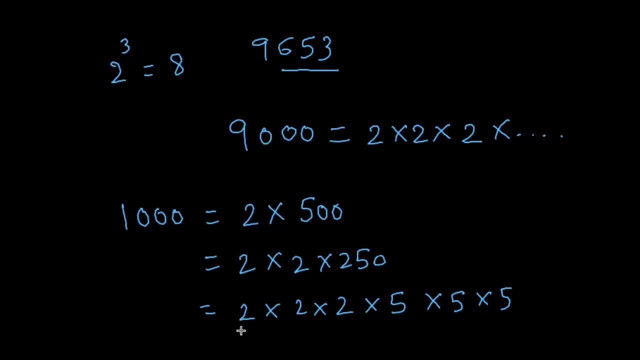 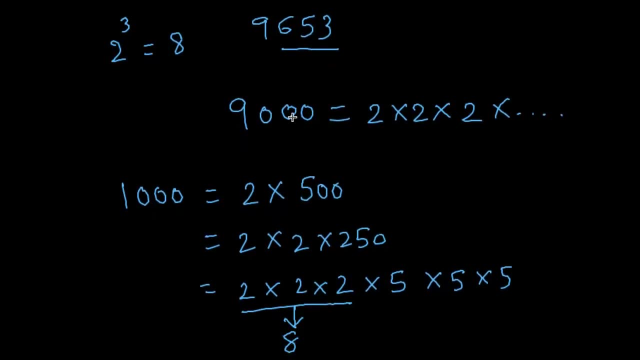 this is the prime factorization et al. The prime factorization of any of the thousands will contain three twos, that is 1: 8.. it will always have one eight in its prime factorization. all thousands will always have one 8 in its prime. 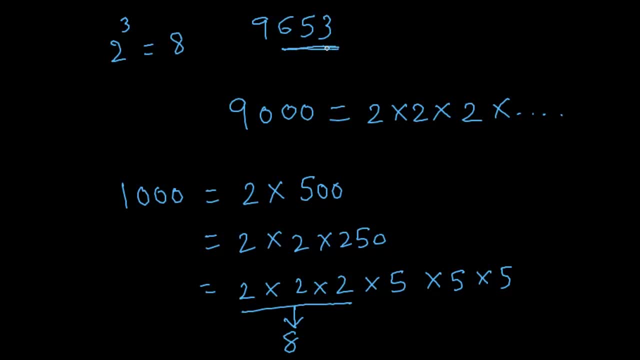 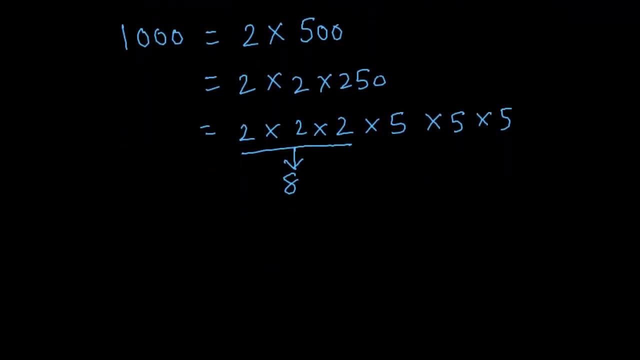 factorization. so the divisibility for 8 always depends upon the last three digits. now we will take the last case, K. This test can be applied to any of the powers of 2, but I will conclude this with this last case, That is, 2 raised to 4 is 16.. The given number is 1,, 9,, 8,, 7,, 5,, 6.. 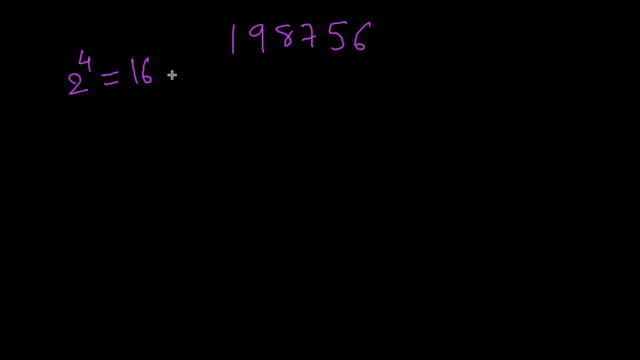 Now, first thing is to divide the number and see if it is divisible. The other way is to check out for last 4 digits. Why last 4 digits? Because all the 10,000s and the higher values would be divisible by 16.. 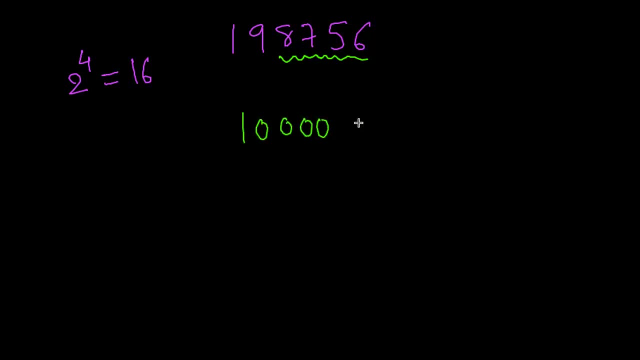 Because, let us say, the number given is 10,000 and 2 into 2,, 4 into 2,, 8, into 2,, 16 and 16, and it will move on. If you want to know the exact prime factorization, we can do it like this: 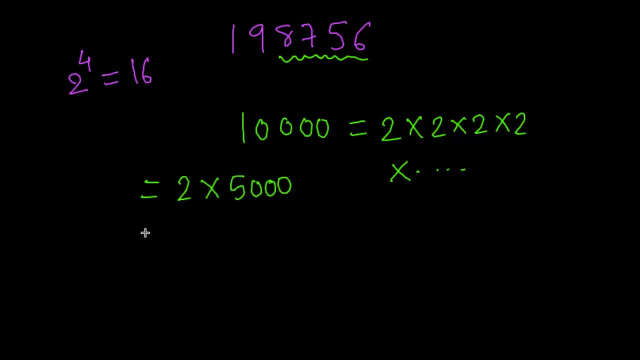 2 into 5,000.. 2 into 2,, 5,000 into 2.. 2 into 2.. And these two zeros would be from 2 into 5, into 2 into 5.. And one more, 25 would be from 5 into 5..